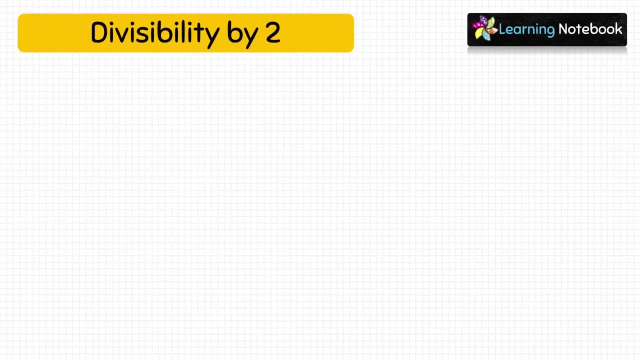 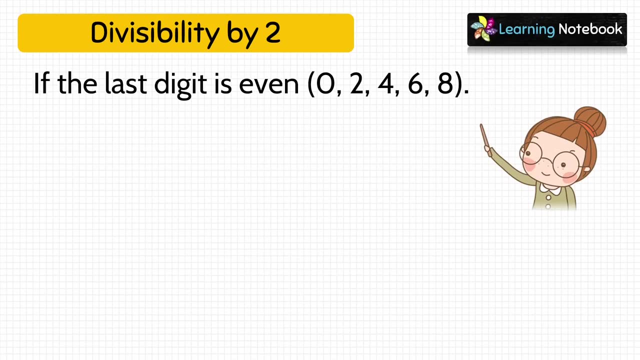 2. If the last digit of a number is even like 0,, 2,, 4,, 6 or 8, then that number is divisible by 2.. For example: 14,, 22,, 36.. Here the last digits are 4,, 2 and 6.. 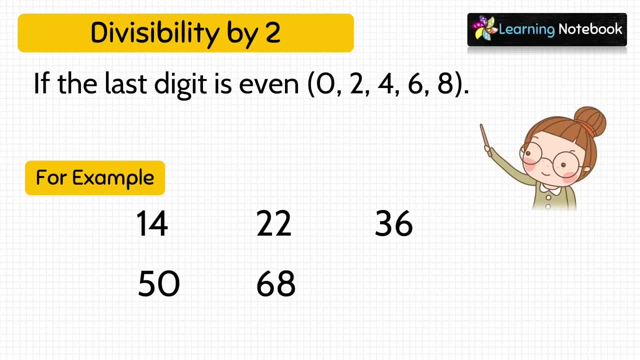 Which are even numbers. So these numbers are divisible by 2.. Similarly, 50 and 68 also have last digit as even. Therefore these two numbers are also divisible by 2.. Now let's see divisibility rule by 3.. 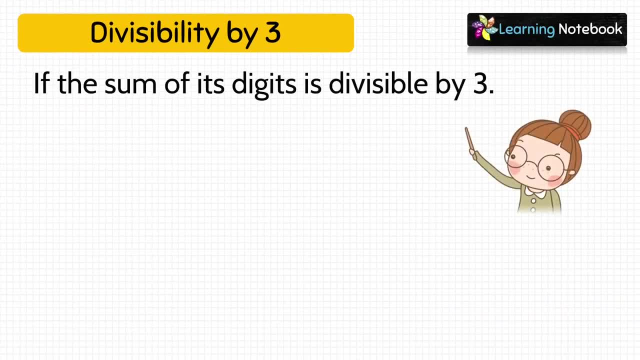 To check if a number is divisible by 2, we have to check the divisibility rule by 3.. To check if a number is divisible by 3,, we will check if the sum of its digits is divisible by 3 or not. 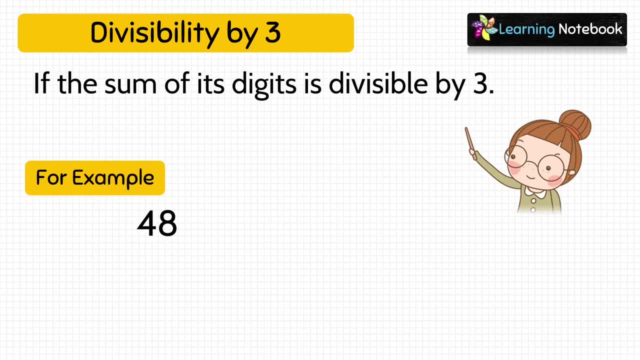 For example, we have to tell whether 48 is divisible by 3. So to check this, we will add 4 and 8. We get 12.. Now we will check if 12 is divisible by 3.. Yes, we know. 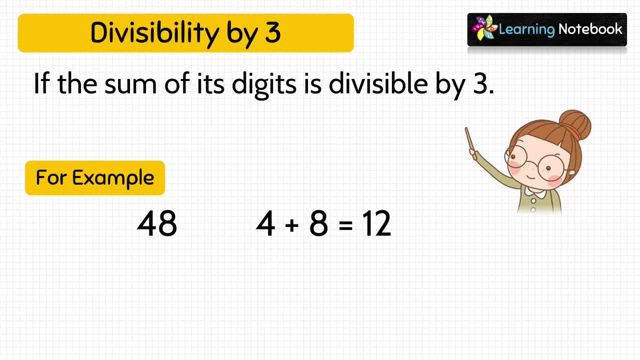 12 is divisible by 3.. Therefore, 48 is also divisible by 3.. Let's take another example. Check if 63 is divisible by 3.. So let's add both the digits: 6 plus 3 equals to 9.. 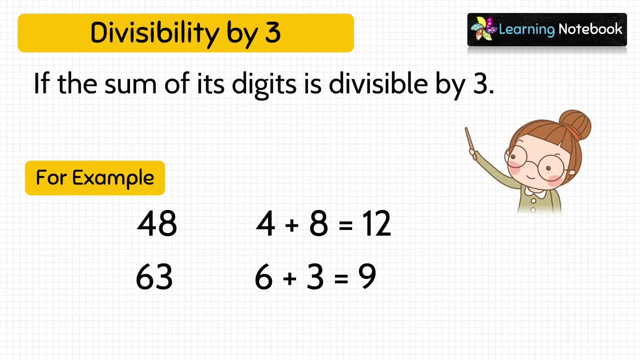 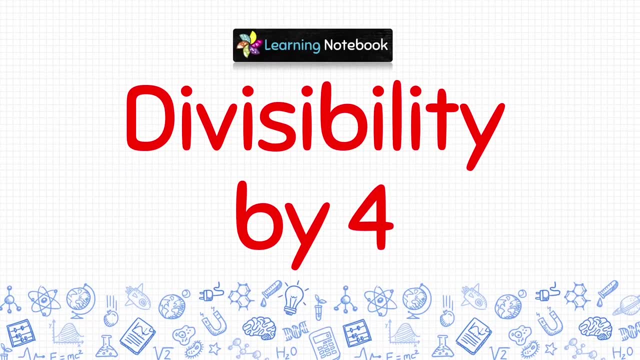 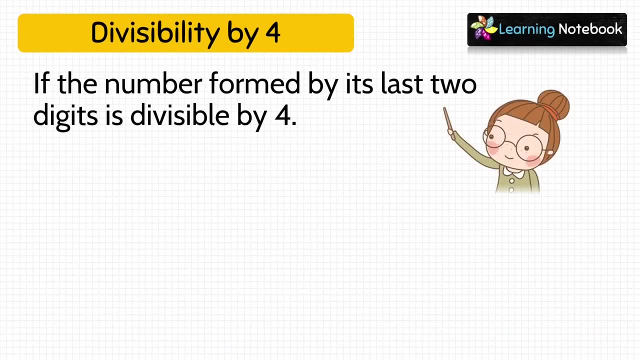 Now 9 is divisible by 3.. Therefore, 63 is also divisible by 3.. Now let's see divisibility by 4.. To check if the number is divisible by 4, we will see if the number formed by its last two digits is divisible by 4 or not. 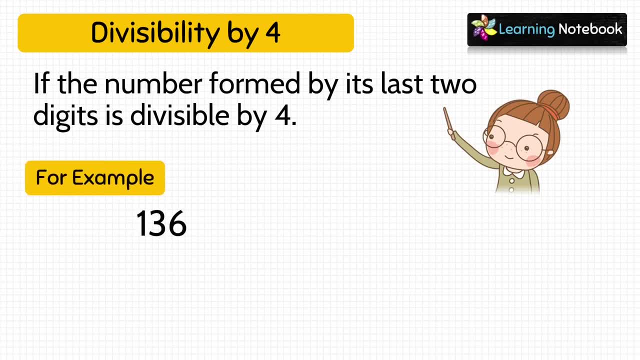 Let's take an example. The number is 136.. So to check if 136 is divisible by 4, we will check if the number formed by its last two digits is divisible by 4 or not. We will check the last two digits, that is, 36 is divisible by 4 or not. 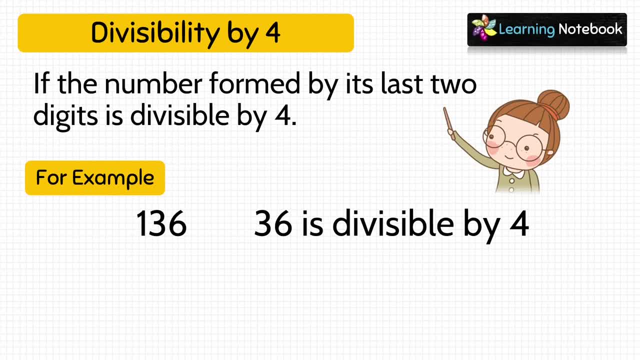 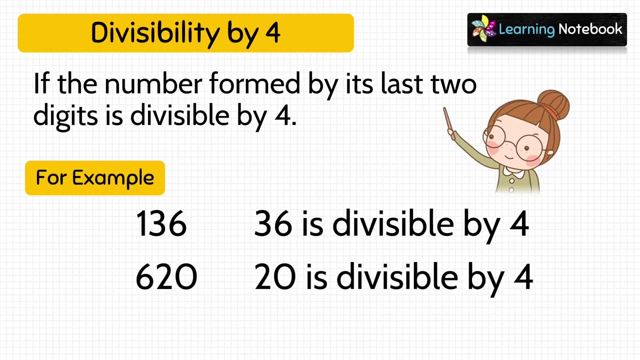 Yes, we know, 36 is completely divisible by 4.. Therefore, 136 is divisible by 4.. Similarly 620.. Here also take the last two digits. the number formed is 20.. The number formed is 20.. The number formed is 20.. 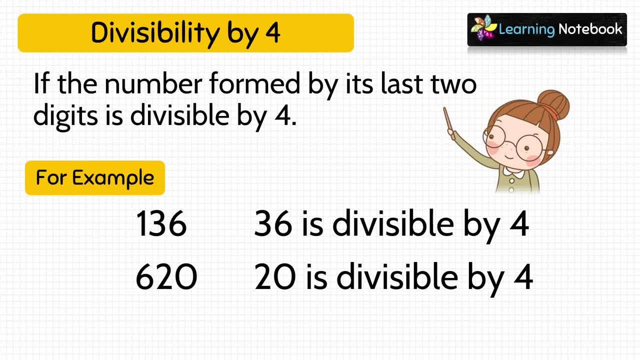 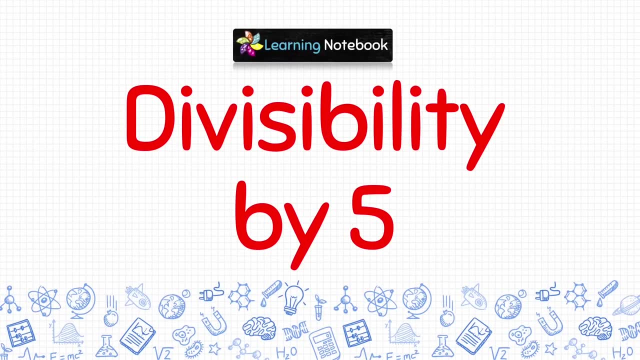 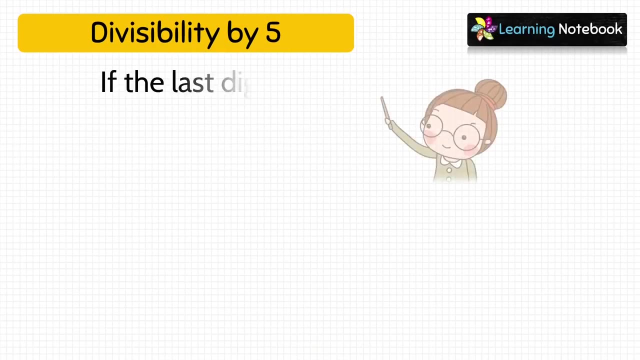 And check if 20 is divisible by 4.. Again, we know 20 is divisible by 4.. Therefore, 620 is divisible by 4.. Now let's understand divisibility by 5. Students, this is very simple. 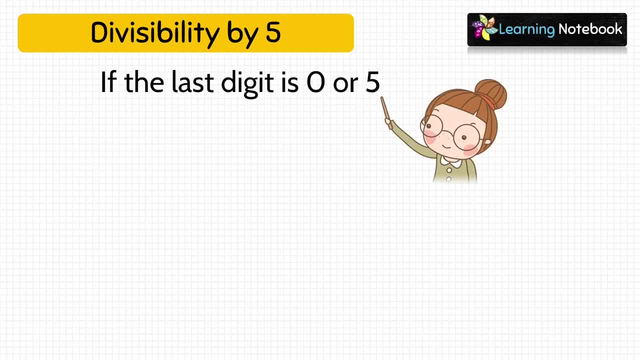 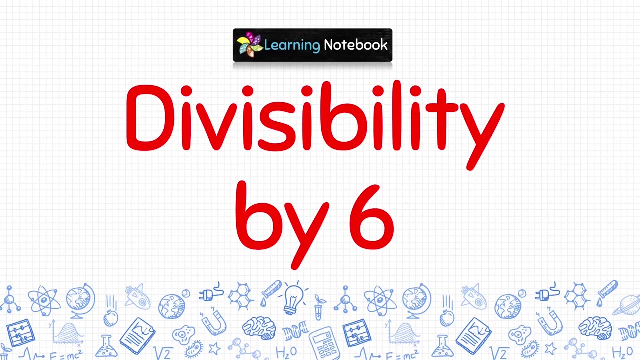 We just need to check if the last digit of the number is 0 or 5.. For example, 140 and 355.. Here the last digit is 0 or 5.. So the number is divisible by 5.. Next is divisibility by 6.. 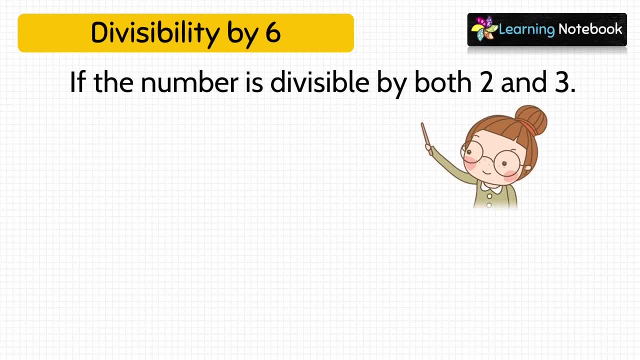 To check if the number is divisible by 5, or if the last digit of the number is divisible by 6,. we will see if the number is divisible by both 2 and 3.. Let's take an example: 336.. This number is divisible by 2 because its last digit, 6, is even number. 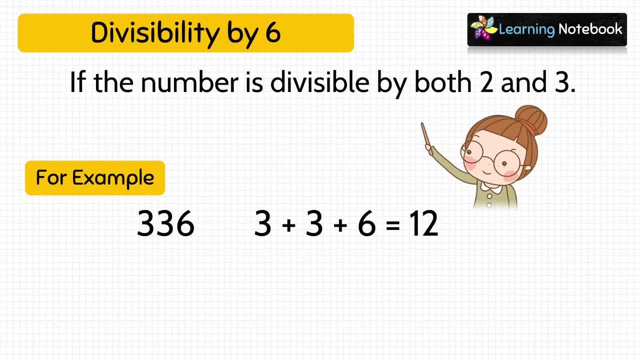 Also, 3 plus 3 plus 6 equals to 12. And 12 is divisible by 3. So 336 is divisible by both 2 and 3. So we can say this number is divisible by 6.. 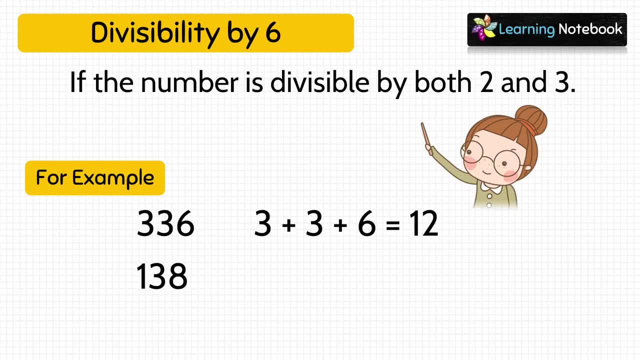 Let's take one more example: 138.. Again, it is divisible by 2, because its last digit is even Also: 1 plus 3 plus 8 equals to 12.. Which is divisible by 3. So this number is divisible by 6.. 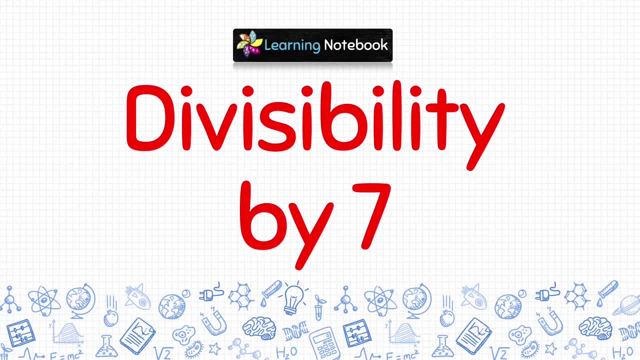 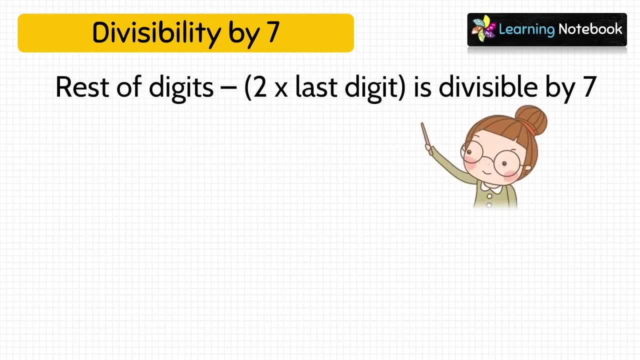 Now next is divisibility by 7. To check if a number is divisible by 7, we will check if rest of digits, minus 2, into last digit, is divisible by 7 or not. Let's see if you examine this number. 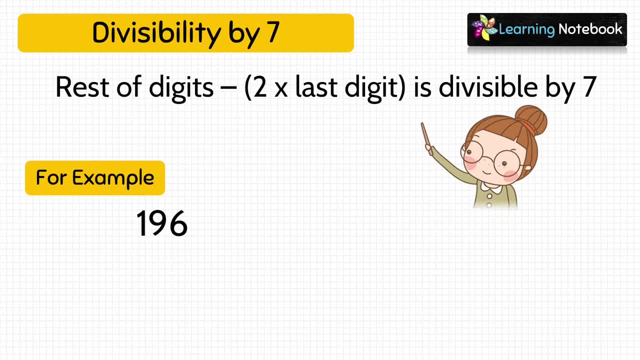 Example 196.. Here last digit is 6 and rest of the digits form 19.. So we will do 19 minus 2 into 6, which is equals to 7.. Now if 7 is divisible by 7, yes, it is. 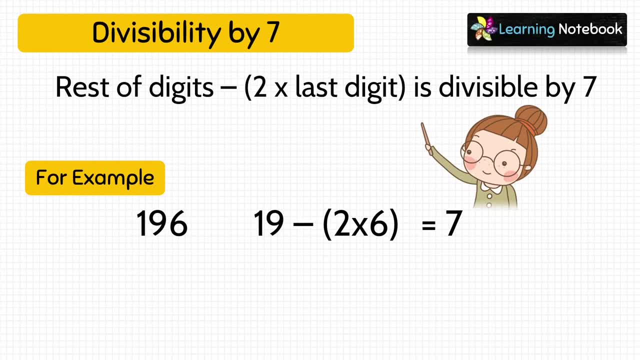 Therefore, 196 is divisible by 7.. Another example is 392.. Here last digit is 2 and rest of the digits form 39. So 39 minus 2 into 2 equals to 35, which is divisible by 7.. 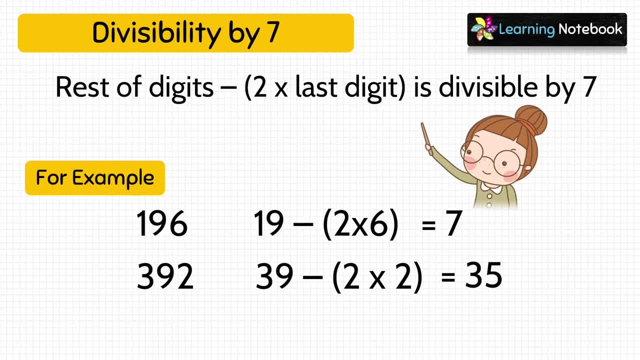 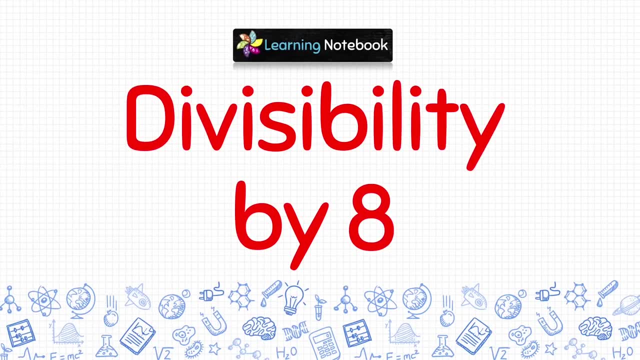 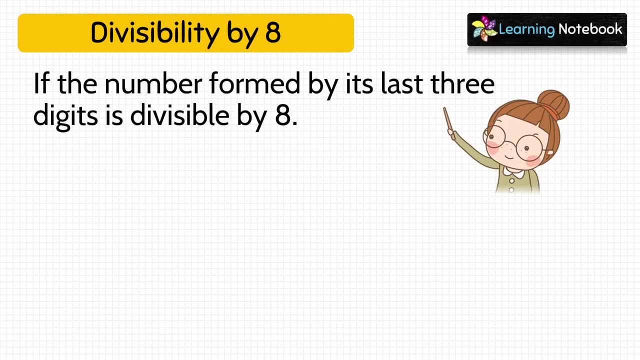 So 392 is also divisible by 7.. Now let's learn about divisibility rule of 8.. To check divisibility by 8, we will see if the number formed by its last 3 digits is divisible by 8.. 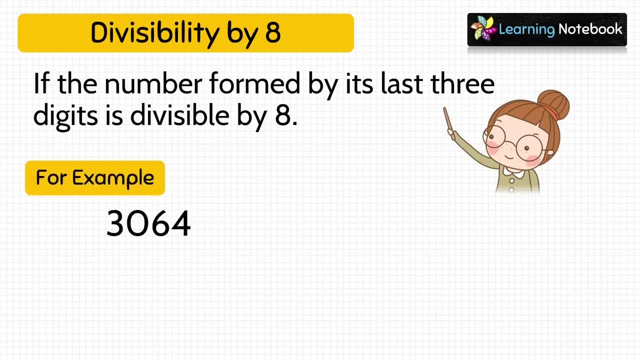 For example 3064.. Here the number formed by last 3 digits is 064 or just 64. Now 64 is divisible by 8.. Therefore we can say 3064 is divisible by 8.. Another example is 1120.. 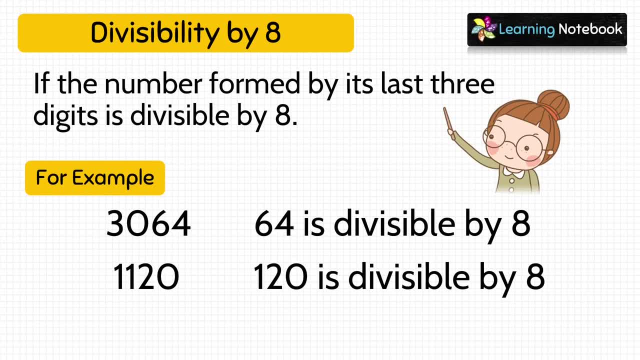 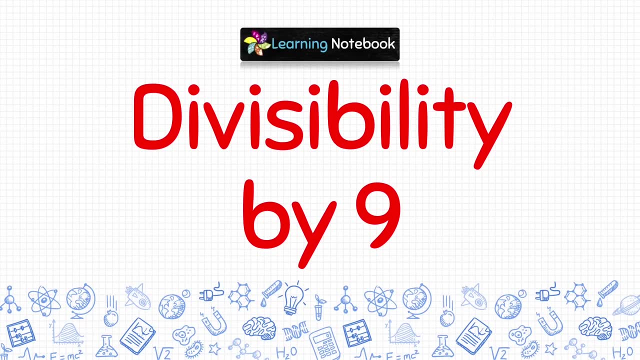 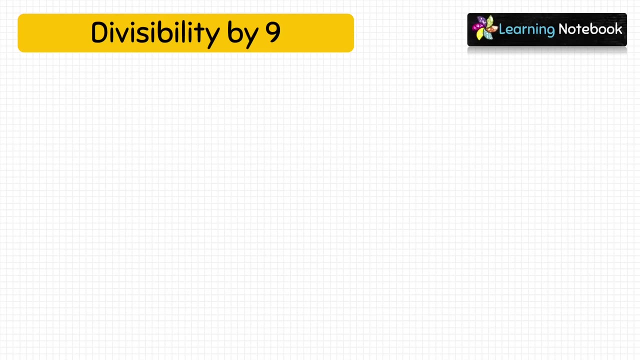 Number formed by last 3 digits is 120, which is divisible by 8. Therefore, 1120 is also divisible by 8.. Next is divisibility by 8. So 9 is divisible by 9. Students: this is similar to divisibility by 3.. 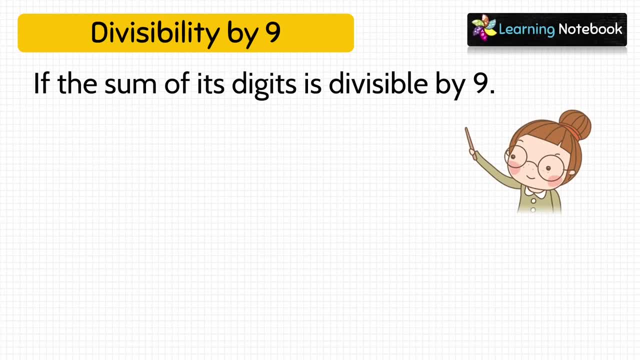 It's just here. we will check if the sum of its digits is divisible by 9.. For example, 108.. The sum of its digits is: 1 plus 0 plus 8 equals to 9, which is divisible by 9.. So 108 is divisible by 9.. 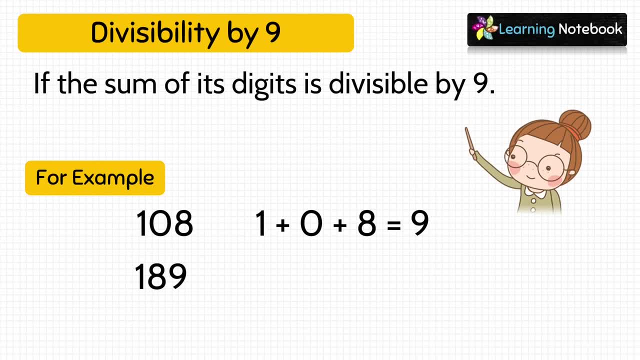 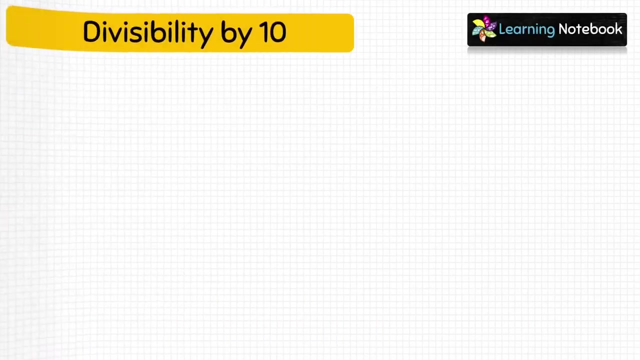 Similarly, 189.. Sum of its digits is: 1 plus 8 plus 9 equals to 18, which is divisible by 9.. Therefore, 189 is divisible by 9.. Next is divisibility by 10.. This one is very simple. 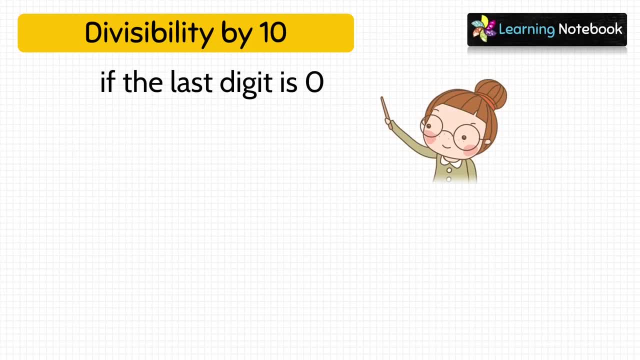 Here we just need to check if the sum of its digits is divisible by 9.. The last digit is 0.. For example, 240 and 550.. Here the last digit is 0. So both the numbers are divisible by 10.. 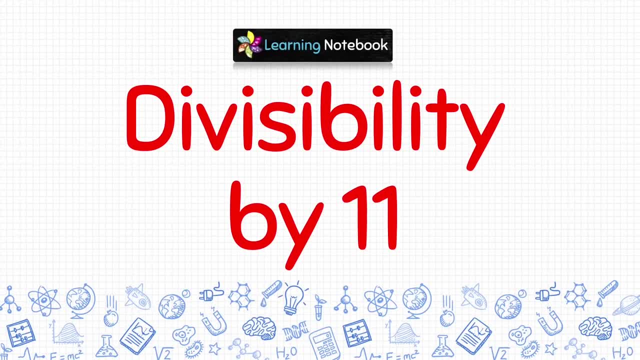 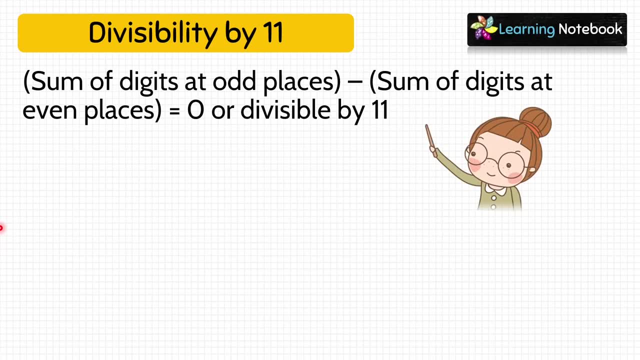 Now the last divisibility rule is divisibility by 11.. Here we need to check that sum of digits at odd place否再 disagrees with 10, the last digit is divisible by 10.. will be divisible by 10.. So the last digit is divisible by 10.. 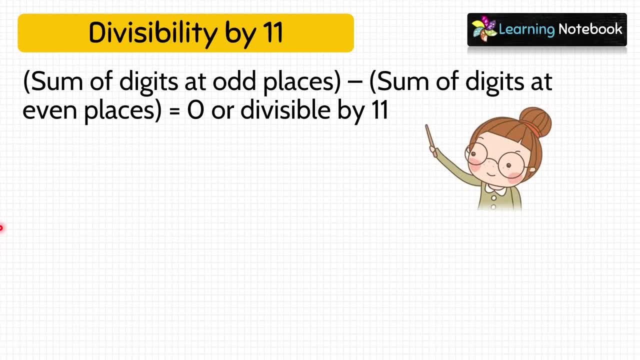 Now, on the other hand, we need to check that sum of digits at odd place, or even less of that. digit places minus sum of digits at even places, should be equal to 0 or divisible by 11. let's take few examples: 616 here. digits at odd places are 6 and 6, and 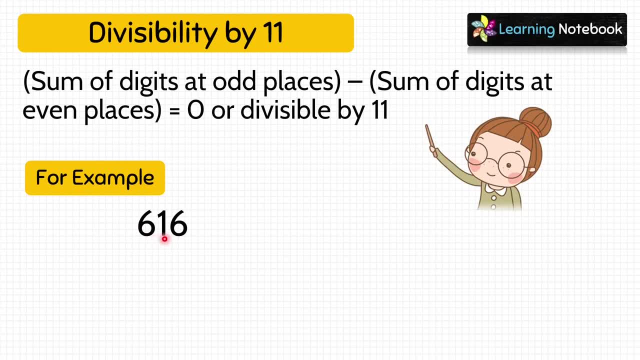 digit at even places 1, so 6 plus 6 minus 1 equals to 11, which is divisible by 11, so 616 is divisible by 11, next 121. here digits at odd places is 1 and 1 and digit at even places 2. 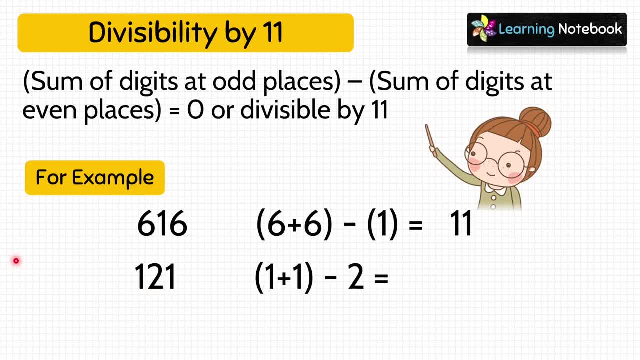 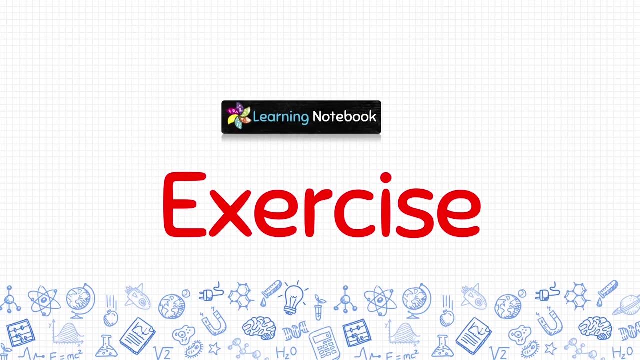 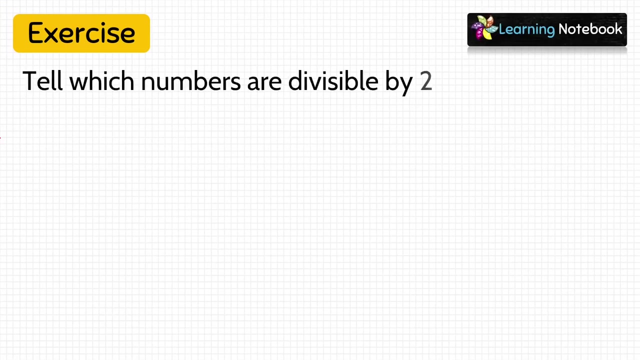 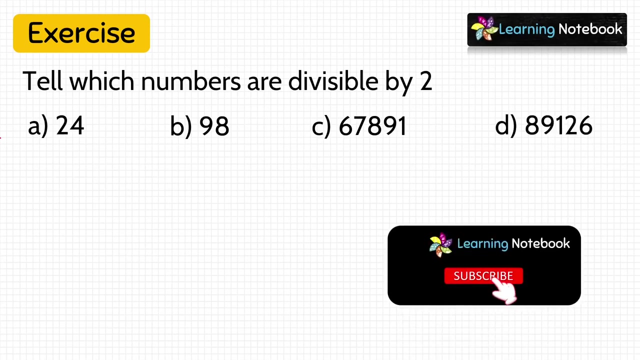 so 1 plus 1 minus 2 equals to 0. therefore, 121 is divisible by 11. so, students, these were the divisibility rules from 2 to 11. now let's practice these divisibility rules with the help of an exercise. question is: tell which numbers are divisible by 2. so we have to tell which. 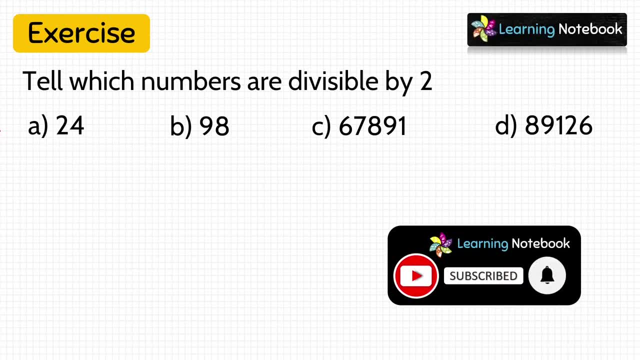 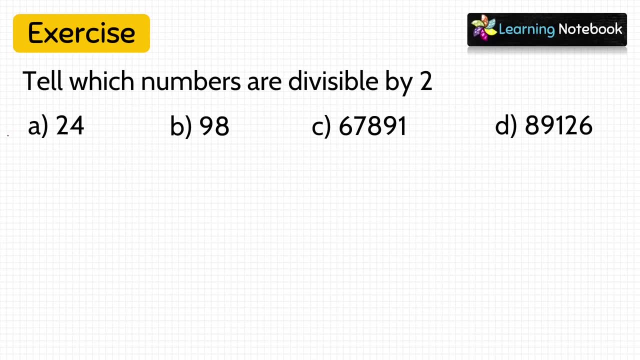 of the following numbers are divisible by 2. we learnt divisibility rule by 2, which says if the last digit of the number is even, then only the number is divisible by 2. so look at this first number, which is 24. its last digit is 4, which is an even number. so 24 is divisible by 2. next, 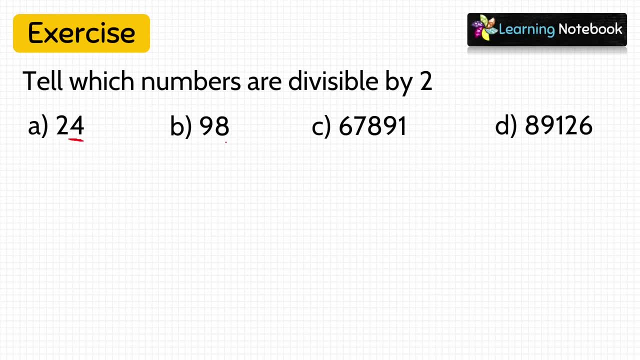 number is 98. last digit is 8, which is also an even number, so 98 is also divisible by 2. next number is 6, 7, 8, 9, 1. its last digit is 1, which is not an even number. so 6, 7, 8, 9, 1 is not divisible by 2. last number is 8, 9, 1, 2, 6, its last. 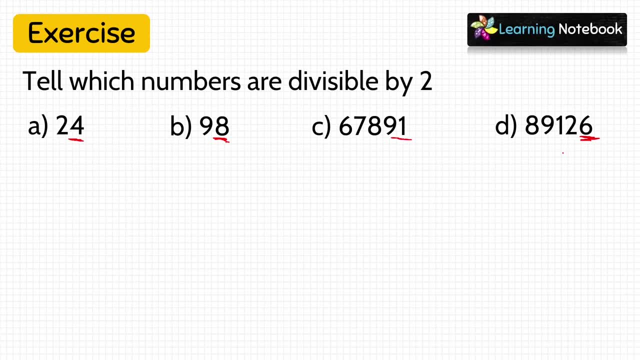 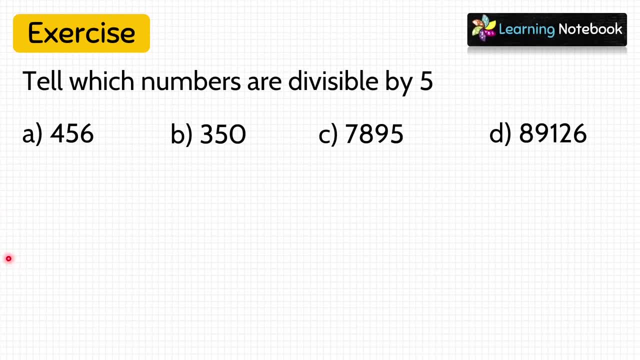 0 or 5, then only that number will be divisible by 5. so let's look at the first number, 4, 5, 6 here. last digit is 6. so this number is not divisible by 5. next number is 3, 5, 0. last digit is 0. 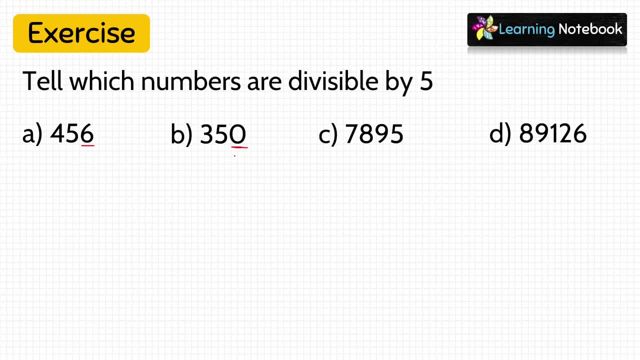 so this means 350 is divisible by 5. next number is 7, 8, 9, 5. again the last digit is 5. so this number is also divisible by 5. last number is 8, 9, 1, 2, 6, 6.. So its last digit is 6.. So this number is not divisible by 5.. So we will write the answer. 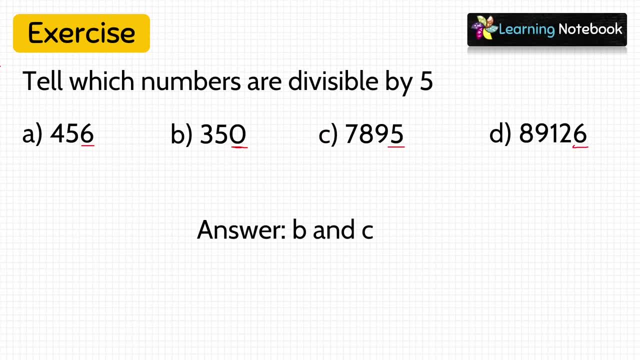 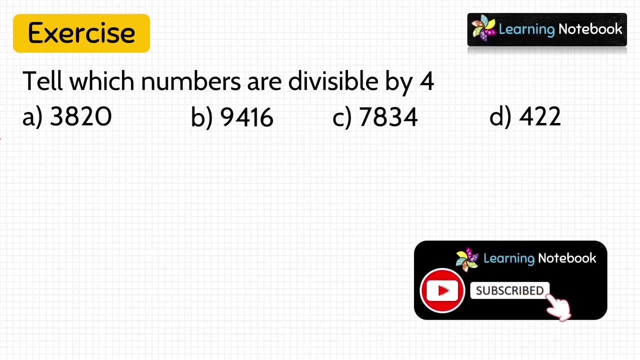 B and C are the numbers which are divisible by 5.. Next question is: tell which numbers are divisible by 4.. So to check if the number is divisible by 4, we will check if the number formed by last two digits is divisible by 4.. So first number is 3820. 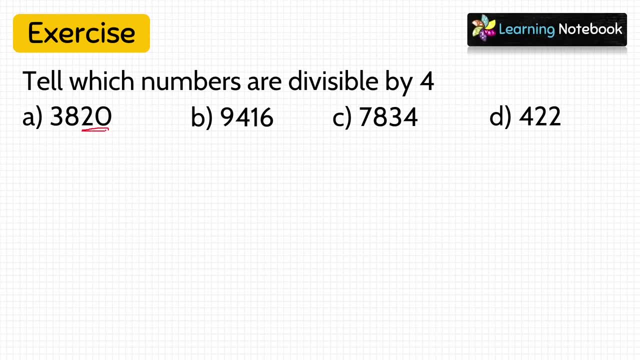 and the number formed by its last two digits is 20 and 20 is divisible by 4.. So it means 3820 is divisible by 4.. Next number is 9416.. So number formed by its last two digits is 16 and 16 is divisible by 4.. So we 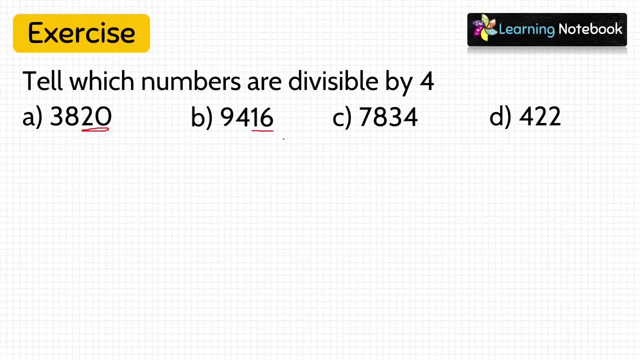 can say: 9416 is divisible by 4.. Let's see the next number, 7834.. Number formed by its last two digits is 34.. Is 34 divisible by 4? No, Then number 7834 is not divisible by 4.. Let's move on to last number, 422.. Number formed by its last two digits is 22, and 22 is. 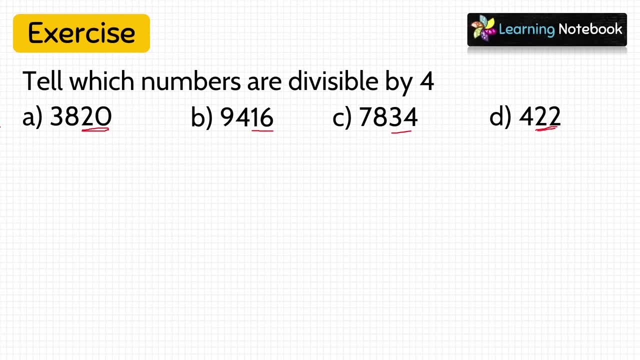 not divisible by 4.. So we can say 422 is divisible by 4.. So we can say 422 is divisible by 4.. So we can say 422 is divisible by 4.. So it means number 422 is not divisible by 4.. So we will write the: 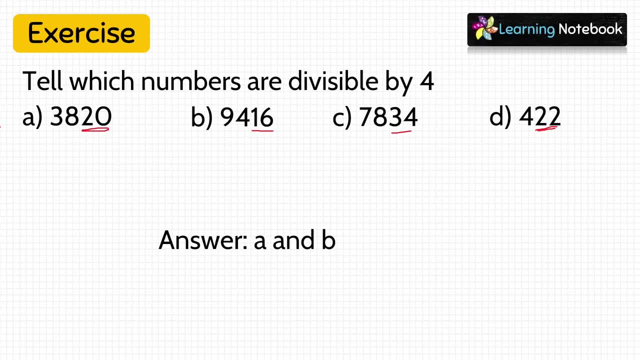 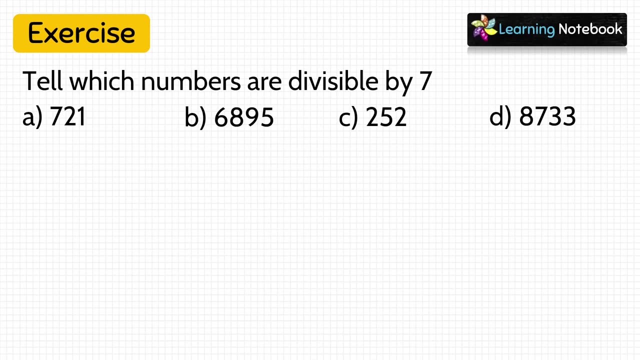 answer A and B are divisible by 4.. Next question is: tell which numbers are divisible by 7.. So to check if the number is divisible by 7, we will check if the number formed by last two digits is divisible by 7. If rest of the digits, minus 2 into last digit, is divisible by 7.. So let's check for. 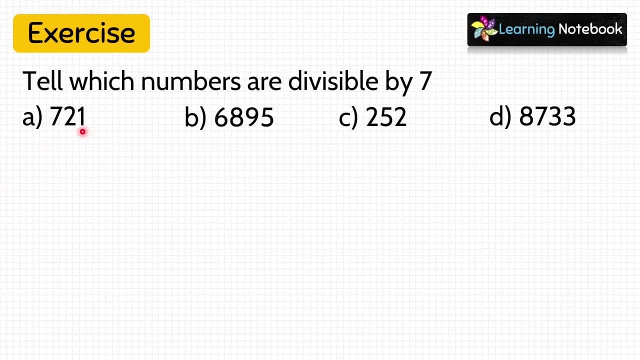 first number, which is 721.. So here we will do 72 minus 2 into 1, which is equals to 70, and we know that 721 is divisible by 7.. So this number, 721, is divisible by 7.. So let's see the next number now. 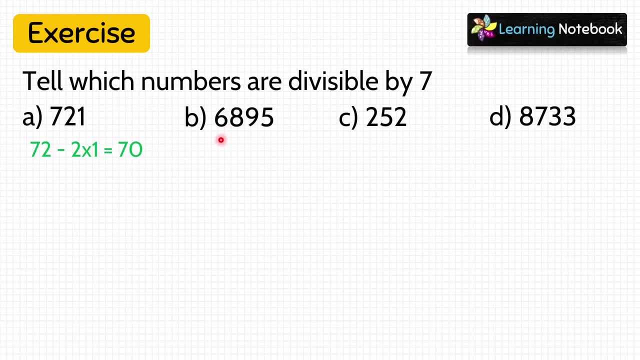 6895.. So here we will do 689 minus 2 into 5, which is equals to 679.. So let's divide this number by 7. And we get 0 as the remainder. So it means 679 is divisible by 7. 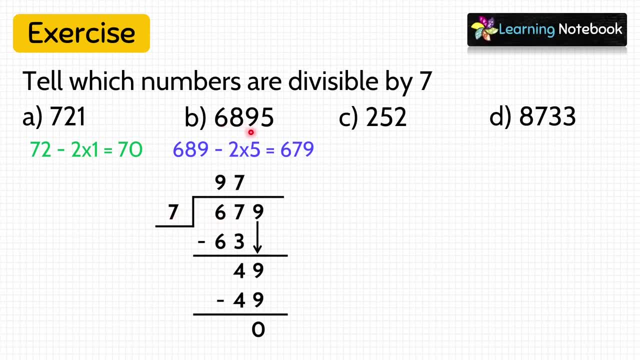 So it means number 6895 is divisible by 7. Next number is 252. So here we will do 25 minus 2 into 2, Which is equals to 21, And we know 21 is divisible by 7, So number 252 is divisible by 7. 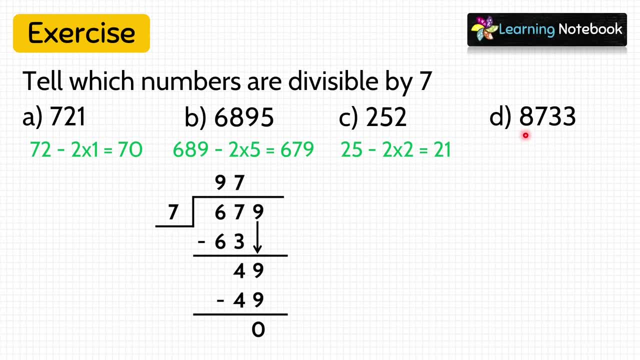 Let's check the last number, 8733. So here we will do 873 minus 2 into 3, Which is equals to 873. So let's divide 867 by 7 And we get 6 as the remainder. So this means number 867 is not divisible by 7. 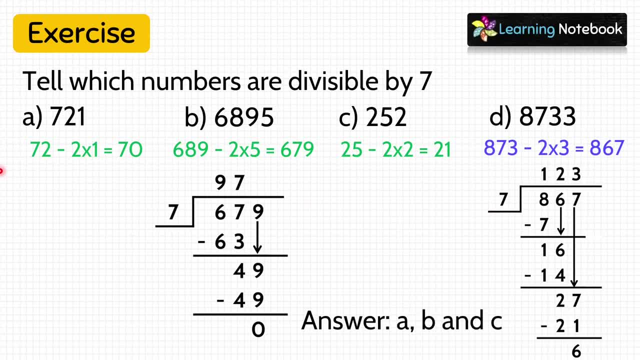 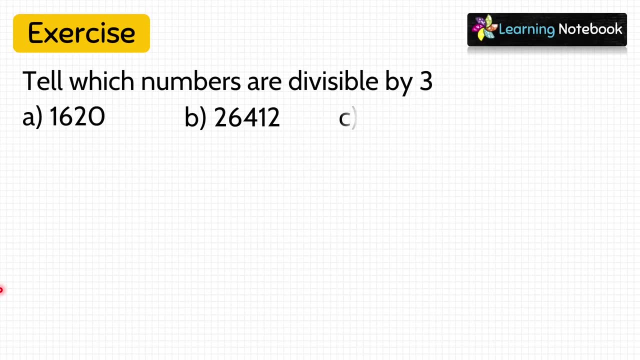 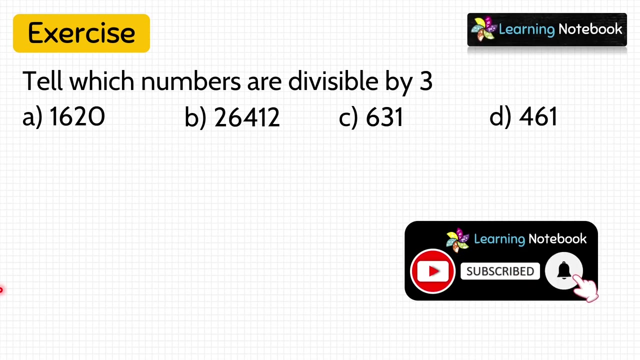 So we can say 8733 is also not divisible by 7. So our answer is A, B and C. Next question is: Tell which numbers are divisible by 3. So here we will check If the sum of the digits of the number are divisible by 3. 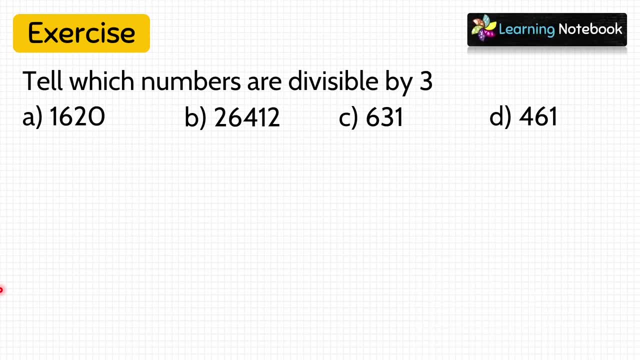 Then only that number is divisible by 3. So let's check for first number, Which is 1620. So let's add All the digits of this number. 1 plus 6 plus 2 equals to 9, And 9 is divisible by 3. 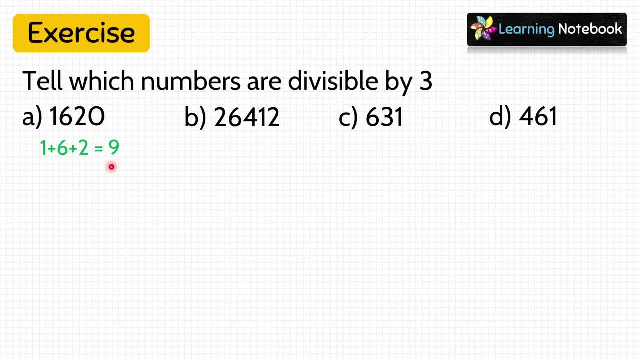 So number 1620 is divisible by 3. Next number is 26412. So we will add all the digits of this number And we get the sum as 15, Which is divisible by 15, divisible by 3.. So this number, 26412, is divisible by 3.. Next number is 631.. So let's add all the. 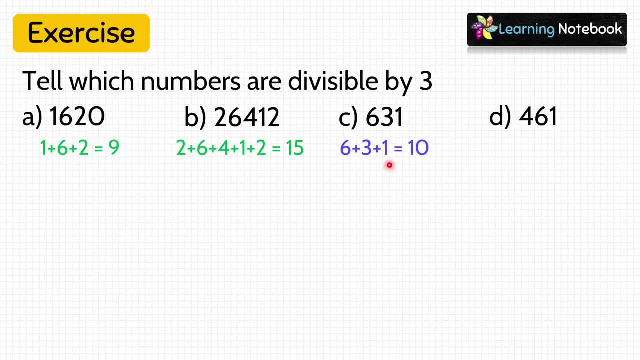 3 digits and we get the sum as 10, which is not divisible by 3.. So we can say number 631 is not divisible by 3.. Last number is 461.. Let's add all the digits and we get the sum as 11, and we know. 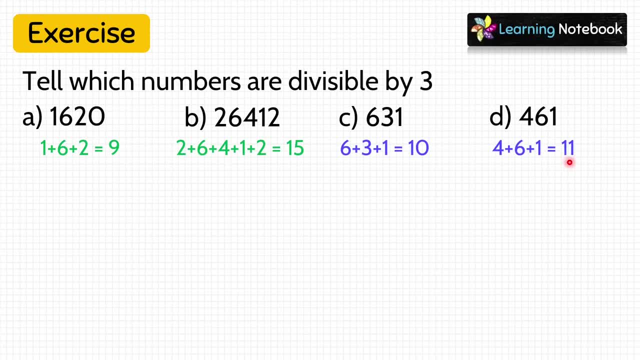 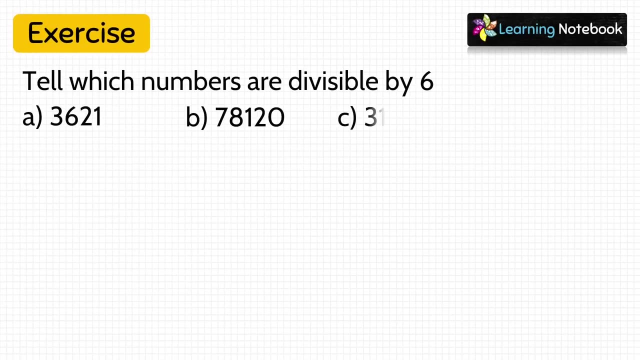 11 is not divisible by 3.. So this number is also not divisible by 3.. We will write the answer as A and B. Now let's do the next question: Tell which numbers are divisible by 6.. So, students, to check if the number is divisible by 6, we have 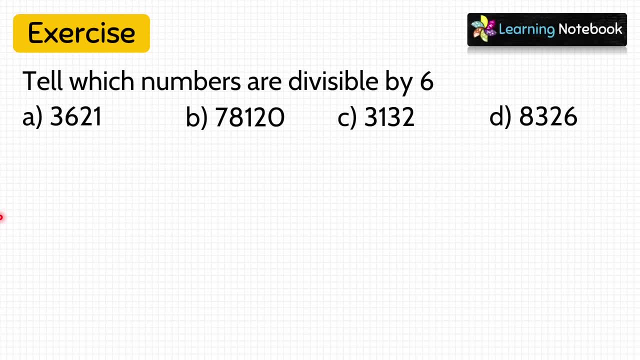 to check if that number is divisible by both 2 and 3.. So first let's check which of the following numbers are divisible by 2.. First number has last digit as 1.. So this is not divisible by 2.. Next number has last digit as 0. So this is divisible by 2.. Next number has last digit as 2.. So this: 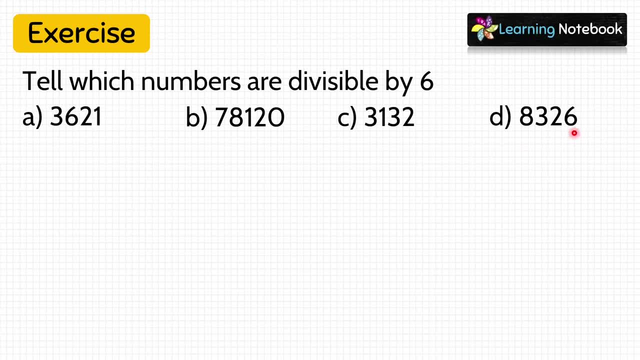 number is also divisible by 2, and then the last number, last digit, is 6.. So this number is also divisible by 2.. Now we know that B, C and D are divisible by 2. So this number is also divisible by 2.. 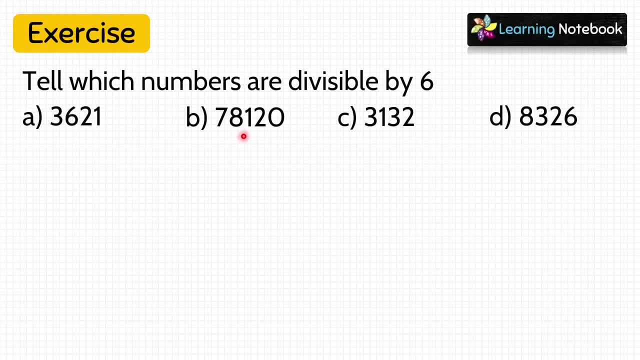 So now we will check if these numbers are also divisible by 3.. So let's add the digits of this number, we get 18, and 18 is divisible by 3. So number 78120 is divisible by 6.. Next, add the. 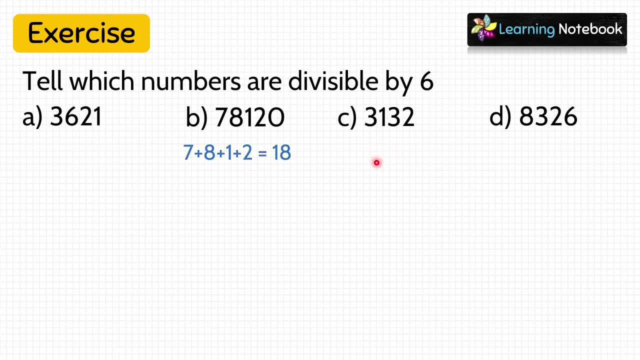 of this number we get 9, and we know 9 is divisible by 3.. So this number, 3132, is also divisible by 6.. Let's check for last number. Add all of the digits and we get the sum as. 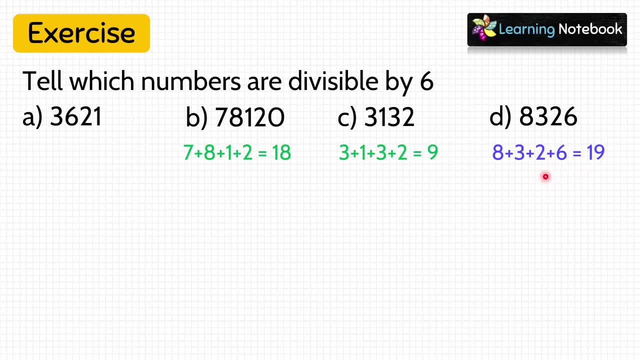 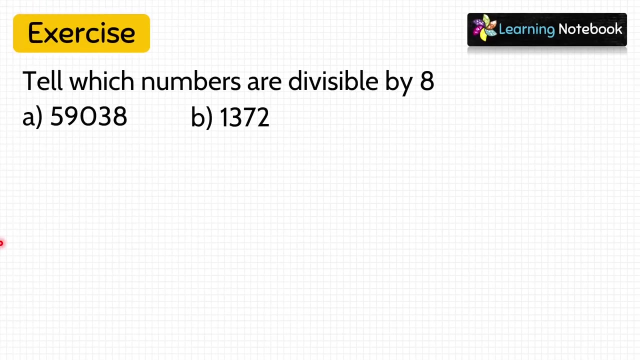 19.. But 19 is not divisible by 3. So this means number 8326 is not divisible by 6.. So our answer is B and C. Next question is: tell which numbers are divisible by 8.. So here we. 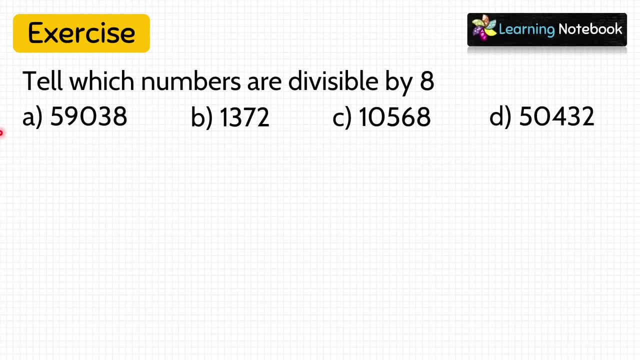 have to check if the number formed by last 3 digits is divisible by 8.. So first number is 59038.. So number formed by its last 3 digits is 38, and we know 38 is not divisible by 8.. So number 59038. 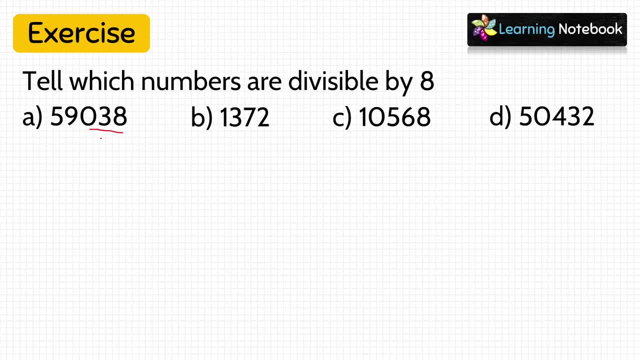 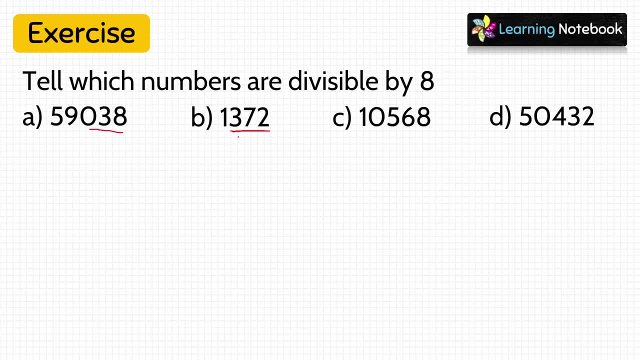 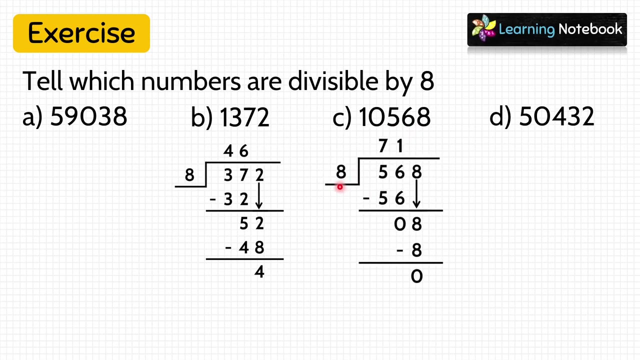 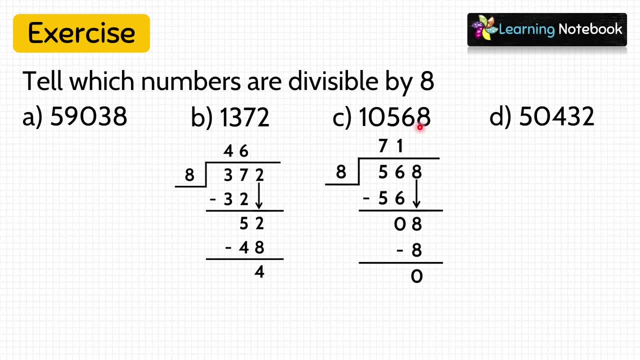 10568 is divisible by 8.. Last number is 50432.. So let's check if number found by last three digits, that is, 432, is divisible by 8.. And yes, we see that, since remainder is 0,. so 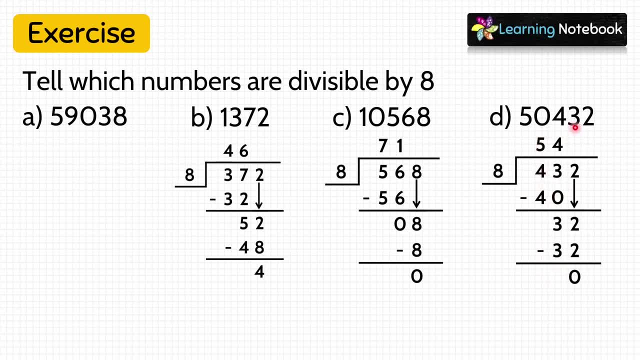 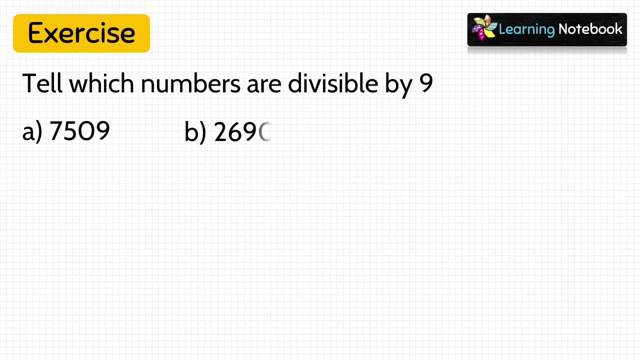 this means number 50432 is divisible by 8.. So we will write the answer as C and D. Now the last question is: tell which numbers are divisible by 9.. So here we will check: if the sum of the digits of the number is divisible by 9, then only that number is. 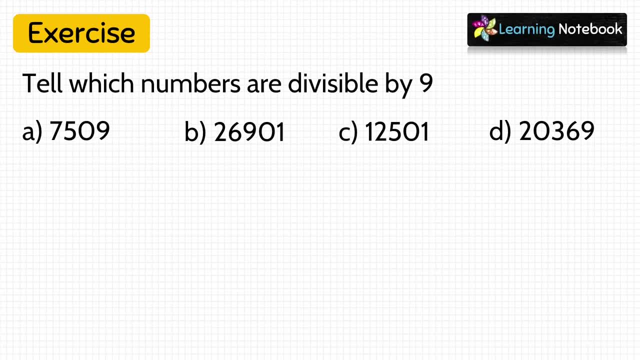 divisible by 9.. So here we will check if the sum of the digits of the number is divisible by 9.. So first number is 7509.. So let's add all the digits, we get 21, and 21 is not. 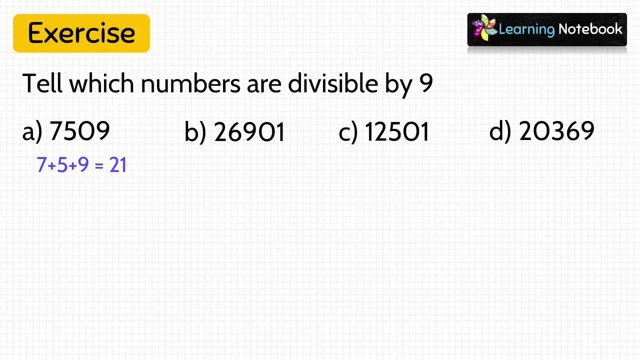 divisible by 9.. So this number is not divisible by 9.. Next, 26901.. On adding all of the digits, we get the sum as 18 and 18.. 9 is divisible by 9.. So this number, 26901, is divisible by 9.. Next number is 12501.. After. 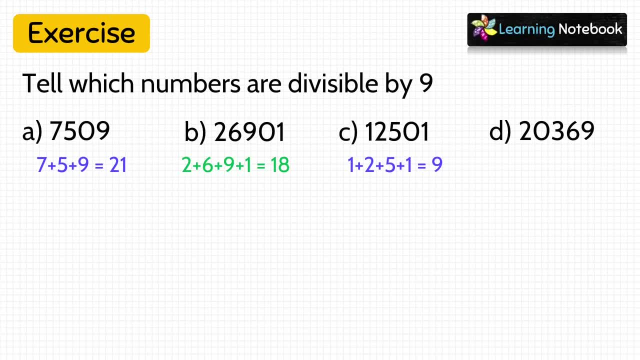 adding all the digits, we get the sum as 9 and 9 is divisible by 9.. So this number is divisible by 9.. Last number is 203.. So this number is divisible by 9.. Next number is 203.. 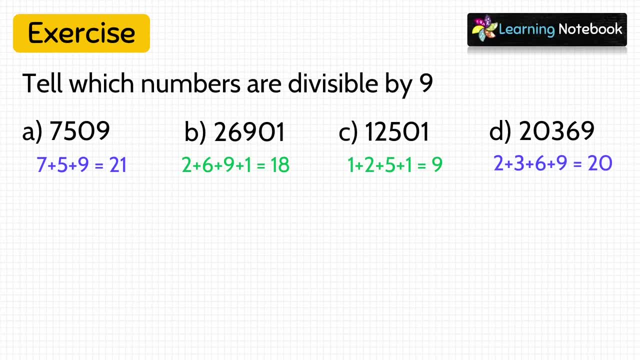 So this number is 269.. Add all the digits and we get the sum, as 20 and 20 is not divisible by 9.. So this last number is not divisible by 9.. So we will write the answer as B and. 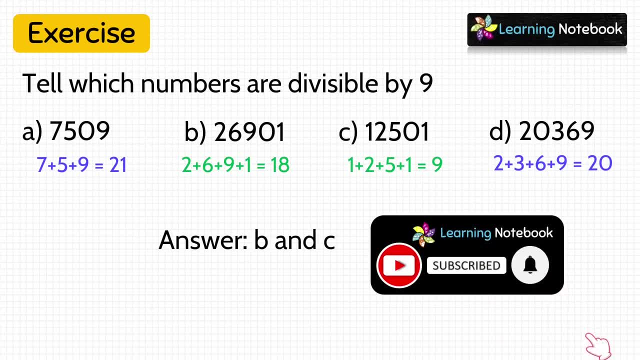 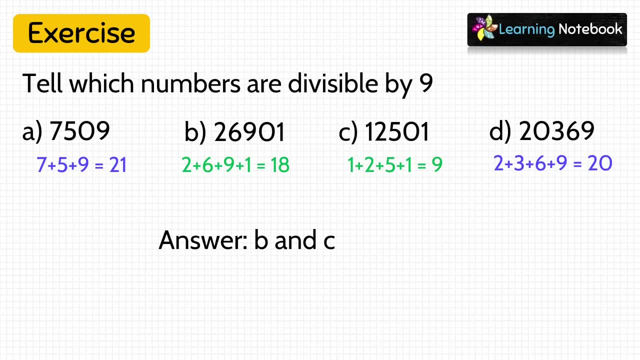 C. So, students, this is the end of our video. Now I am sure you have learnt and understood all the divisibility rules From numbers 2 to 11, do practice these divisibility rules and watch my other videos too, and share. 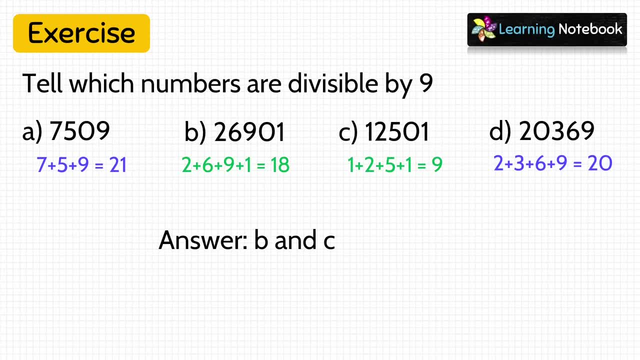 my channel and my videos further. Thanks for watching. See you in the next video. Bye-bye.